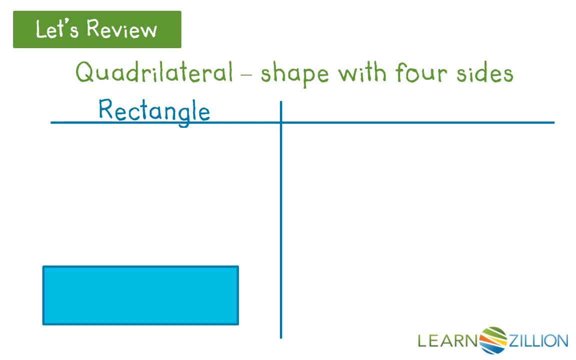 Let's take a look at a rectangle. A rectangle has four square corners. It has four sides. Opposite sides are the same length, The top and the bottom are the same length and the end sides are the same length. Let's take a look at a square. 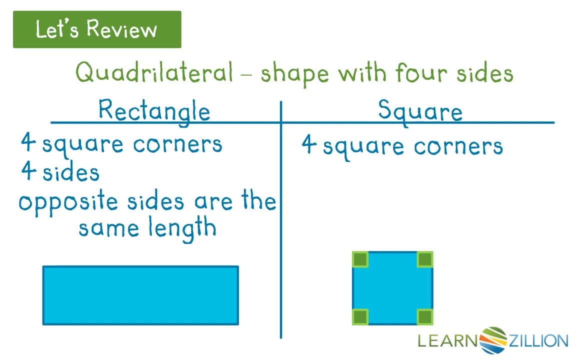 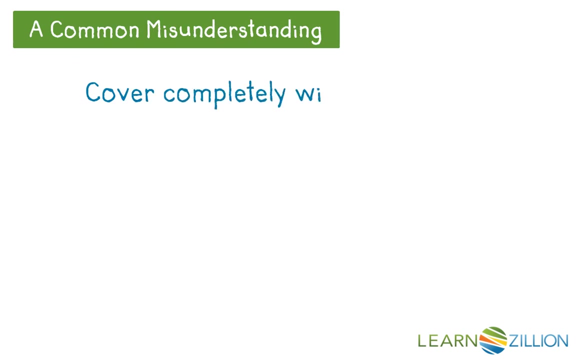 A square has four square corners. It has four sides. All sides are the same length. If we look at all these attributes, the only one that is different between these two quadrilaterals is the length of the sides. When we have a shape and we are going to cover it completely, we have to make sure there is no overlap. 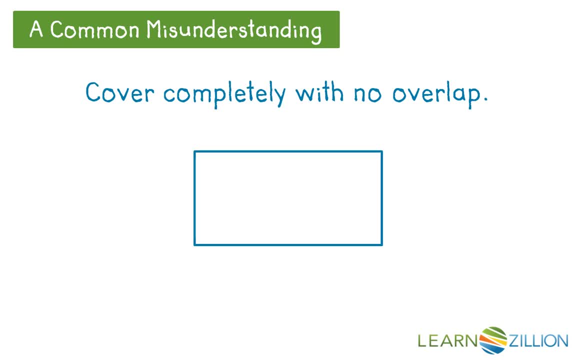 For example, here we have a rectangle and I want to cover it with pieces of paper. I would place this paper and then the next paper, But we notice that there is an overlap. What does that mean? Here we have an overlap. That means that one piece of paper is on top of the other. 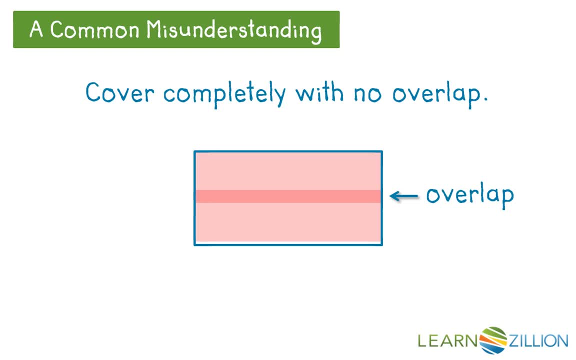 They're not next to each other touching, but one is on top of the other. We also notice that we have a section here that is not covered. It's important that we cover the entire rectangle, So we would have to do the following: 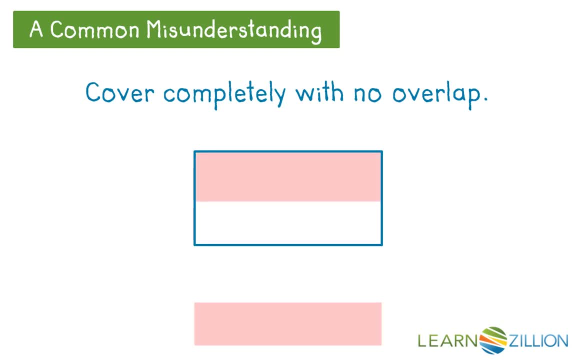 We would take one piece of paper and slide it and then take the other piece of paper and slide it right next to each other And we notice that there is no overlap and there is no section that is not covered. Partition means to separate something into sections. 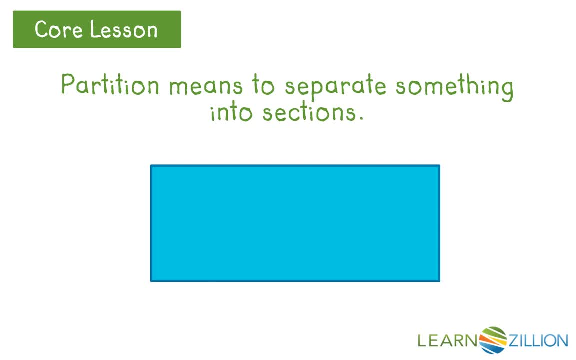 For example, this rectangle. I could draw lines to go through it And I would be partitioning into sections. Today we are going to use squares. Squares are going to be placed on top of the rectangle to partition the rectangle And we are going to count to see how many squares it takes to cover the rectangle, with no overlap.